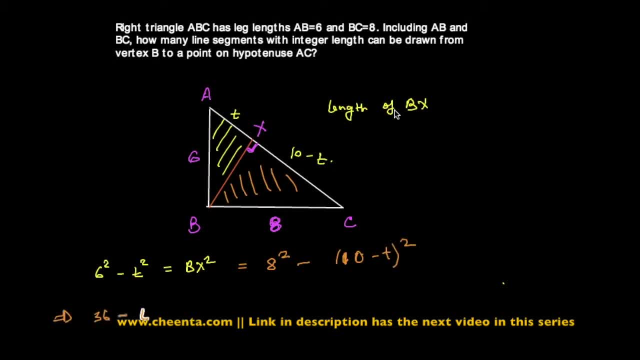 this equation, you get 36 minus T square equal to 64 minus 100, plus T square minus 20 T. so you get 36 minus T square equal to 64 minus 100, minus T square plus 20 T. so clearly negative T square, negative T square will cancel and. 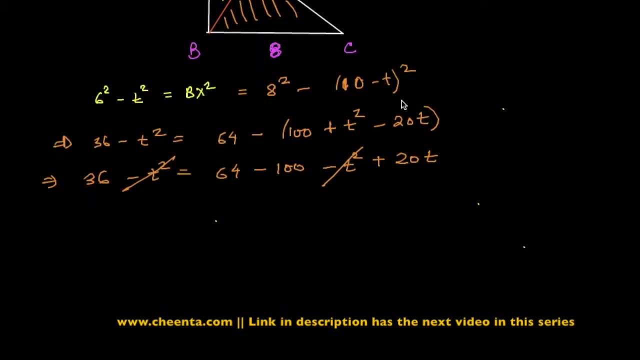 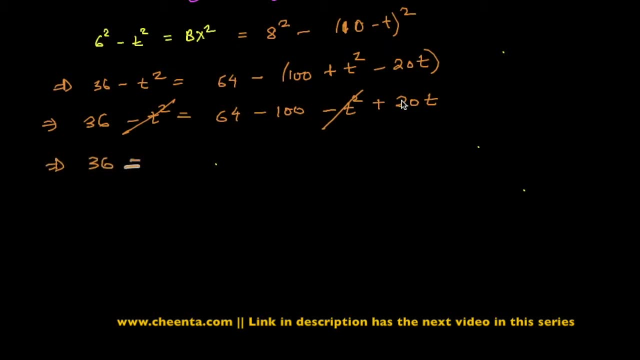 we have 36 equal to negative 36 plus 20 T, which means T equals to 72 by 20. so if this is the value of T, which is, you can simplify it, but we really want to find out BX. so so then we can find out BX. 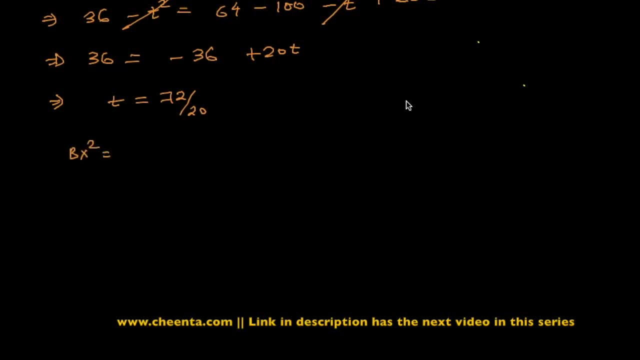 so we got anything that we need upgraded. we can get rid of BX. we don't actually need to sum that. I think I say alright, is reactivity of which one? so we need this value, and then we get our 3.70. so let's do a little bit of. 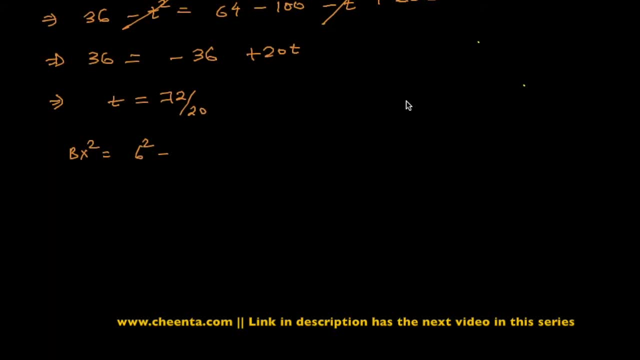 question about wages, next values: ok, vamos to find out. dynamic value of BX. so actually, how many times you get? we mean, how did you average? or usually, what average have you got? we have abouttat wires. There is a number of ways of computing this. Let me just do one. So 6 minus 3.6, 6 plus 3.6, and this happens to be 9.6 and this happens to be 2.4, and you can easily compute 9.6 times 2.4.. 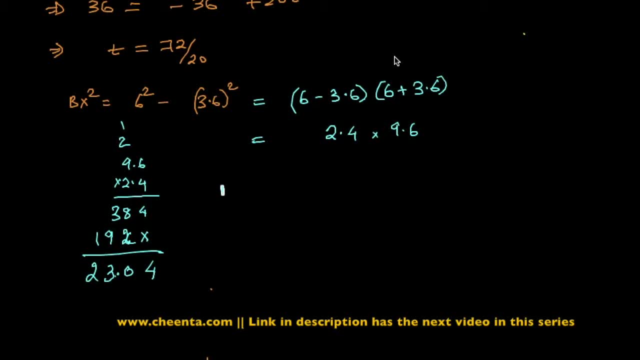 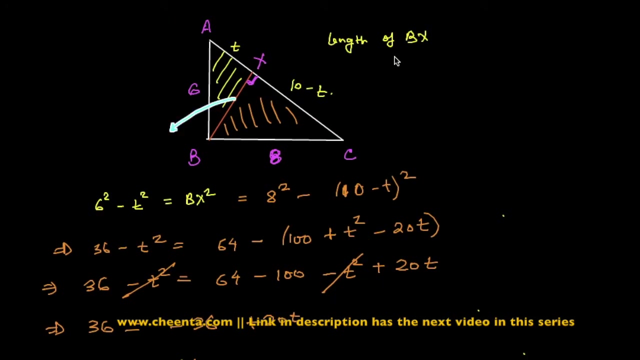 So it's so. bx is approximately square root of 23.04, which is certainly less than 5, but more than 4.. So this value of bx down here is somewhere between 4 and 5.. Now this is the part where you will need intermediate value property. 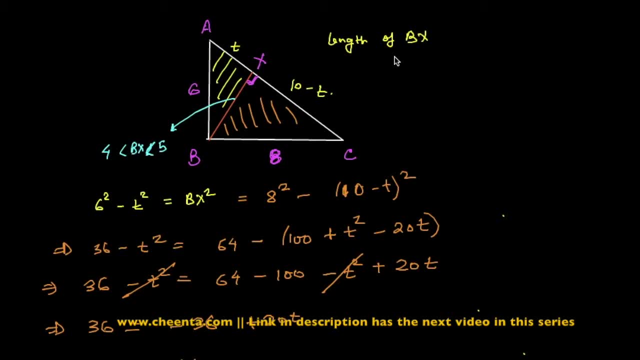 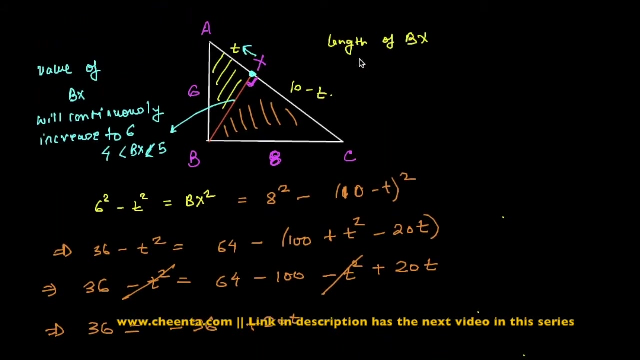 If you drag bx or the point x to the left, notice that it will continuously so. value of bx or the length of vx, value of bx will continuously increase to 6, right, It will continuously increase to 6.. So it will start from 4 points something, and then it will increase to 6 means somewhere in between. 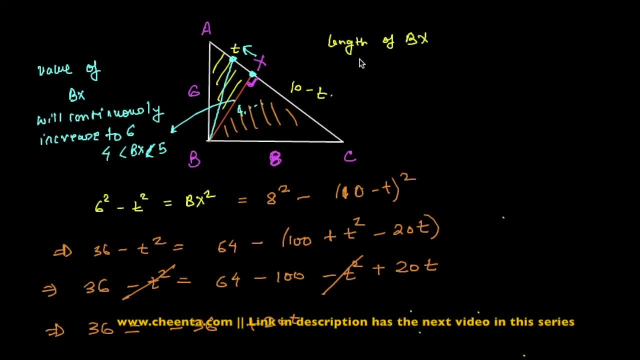 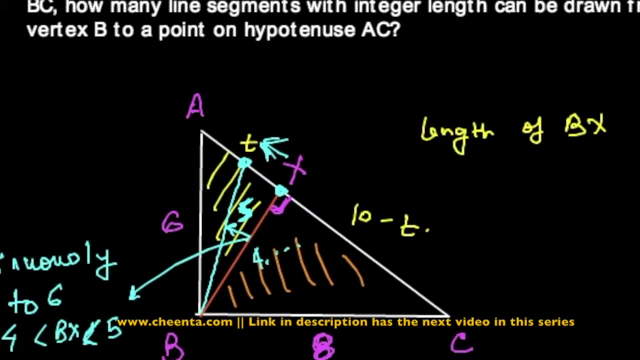 since this increase is happening continuously, it will be achieving the value of 5.. bx is the shortest one from b to ac, so it will gradually increase. the length of bx will gradually increase as x moves towards a, And somewhere in between a and x it will achieve the value of 5.. 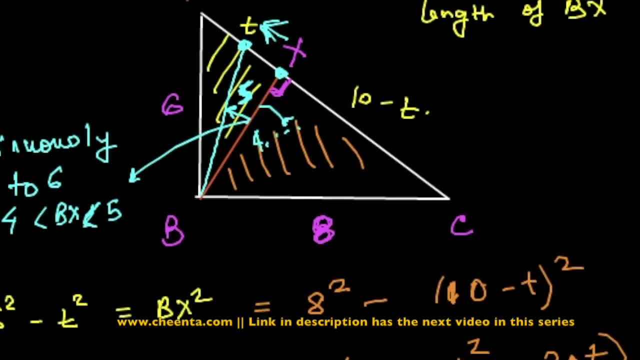 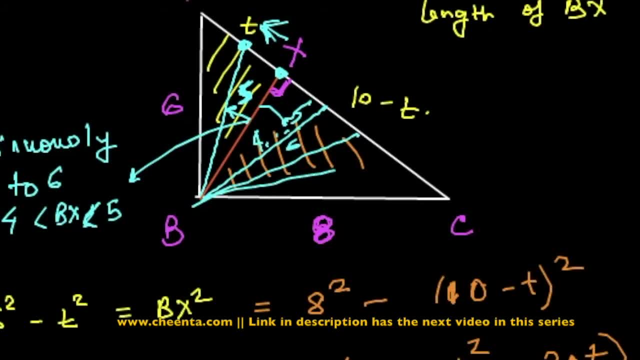 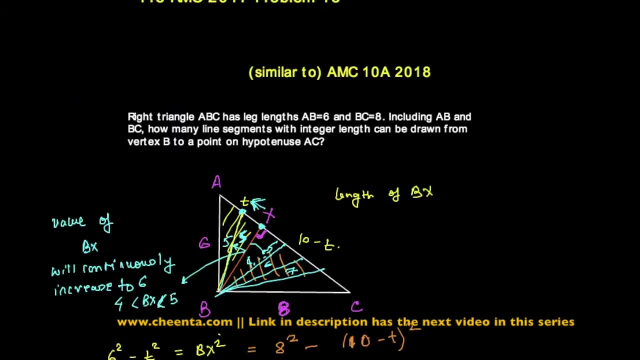 Similarly, as it moves rightward, it will start and increase from 4 point something, and then it will achieve the value of 5.. 6, then 7 and then finally to 8. so we have got how many straight lines which are integer lengths? now we have this one, 5 to the left of BX, and then we have 5.